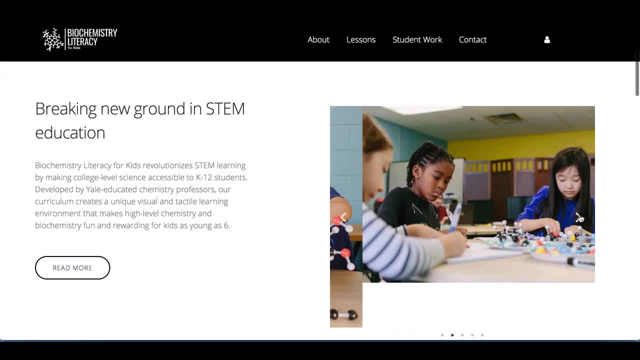 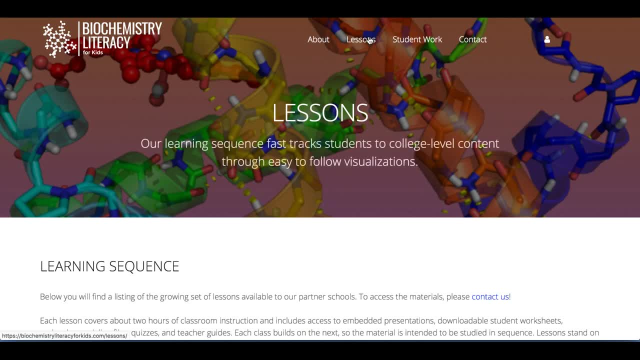 Biochemistry Literacy for Kids is an online curriculum system used by K-12 teachers to bring college-level science into their classrooms. Teachers access our custom materials through our website. We have created thousands of slides that present advanced concepts in a kid-friendly way. 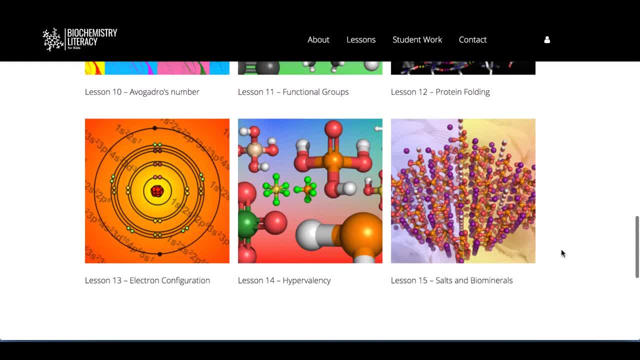 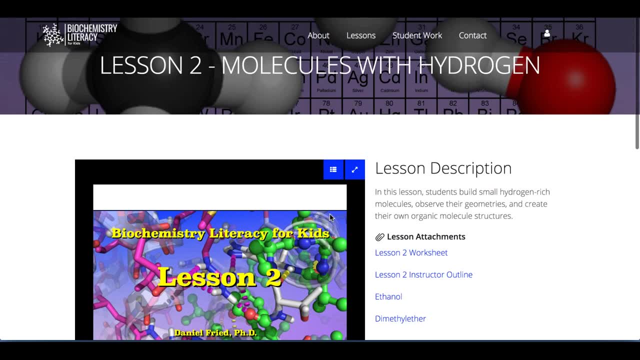 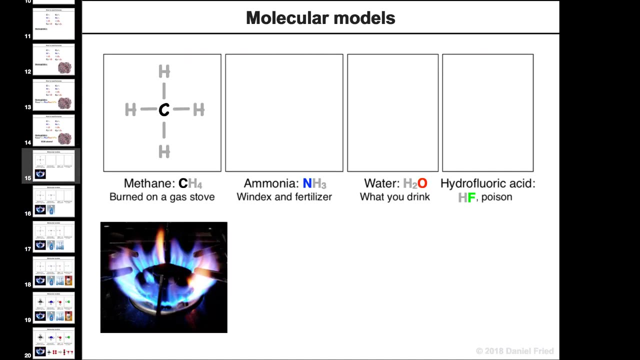 Foundational lessons cover atoms, bonding and the periodic table. Advanced lessons cover college biochemistry units like protein folding and genetics. Let's look at an introductory lesson. Teachers open the embedded presentation and use it just like PowerPoint. This lesson teaches atomic color coding and molecular geometry. This visual approach makes traditional chemistry topics like 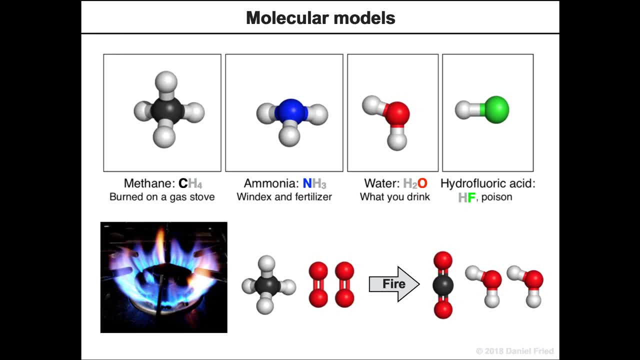 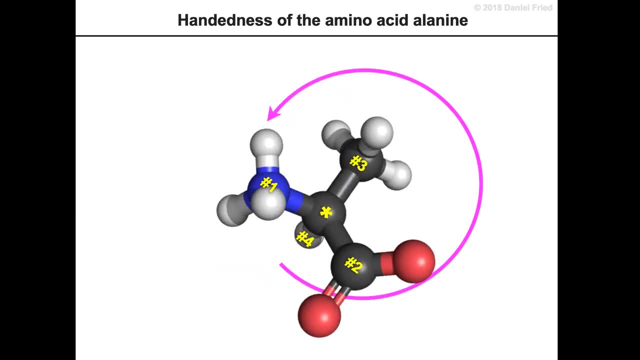 balancing equations much easier and more interesting. Let's skip ahead to a more advanced lesson and see an animation about molecular handedness. Amino acids in our body are left-handed- like this one. These animations allow students to learn about the biological world to a depth. 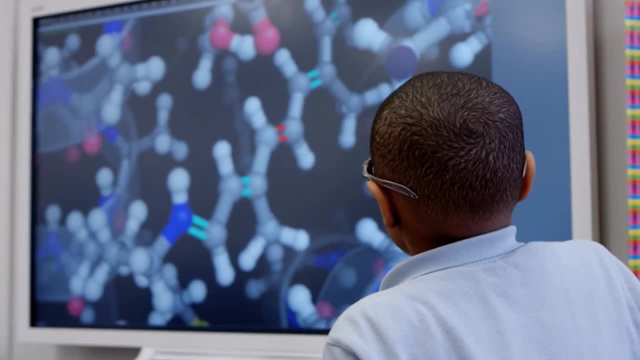 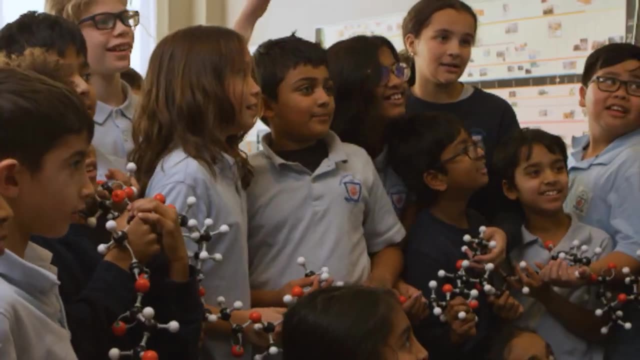 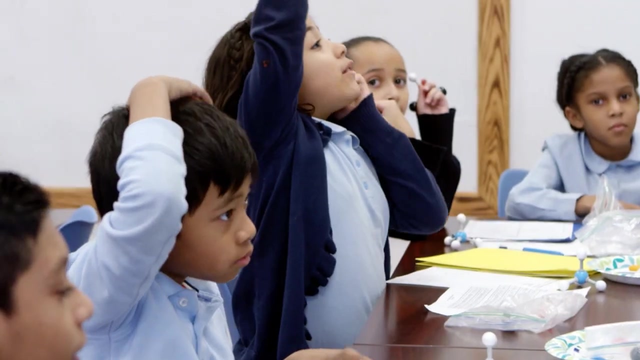 that is unimaginable. Our digital lessons set the stage for physical model building activities like this one, where the class worked together to build a biodegradable plastic polymer. Despite being far above grade level, our lessons inspire and motivate students and give them a wealth of practical 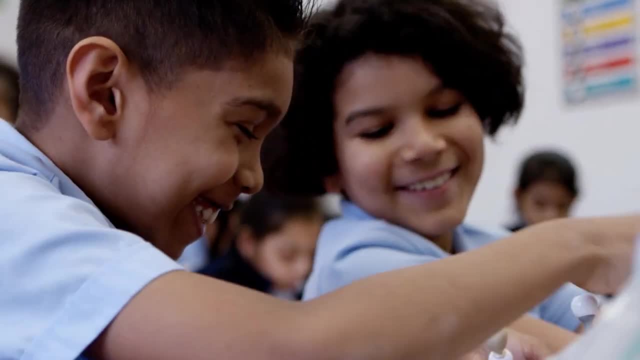 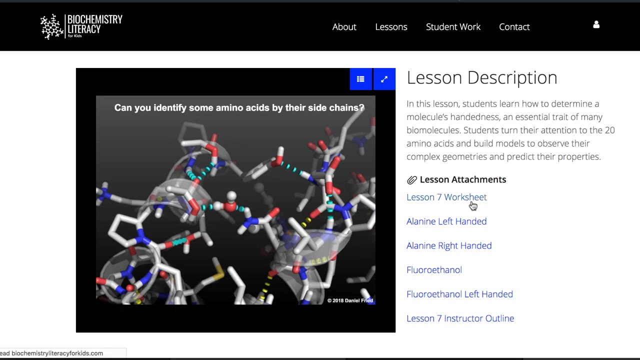 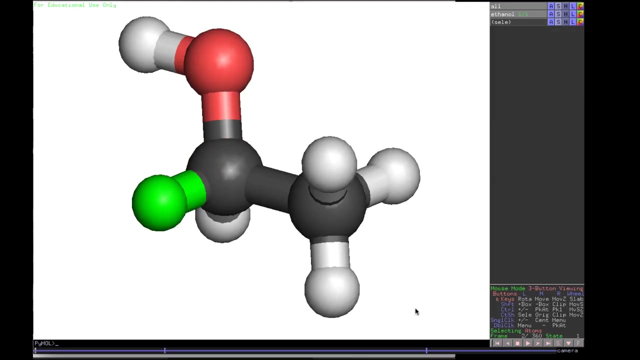 knowledge that most people never get to learn. Our assessment data shows that kids really do achieve college-level learning outcomes from our programs. Each lesson on our page also contains downloadable student worksheets and a lot of information on how to use them. In addition, our lessons are linked to each lesson page and can either be presented by the teachers or used by 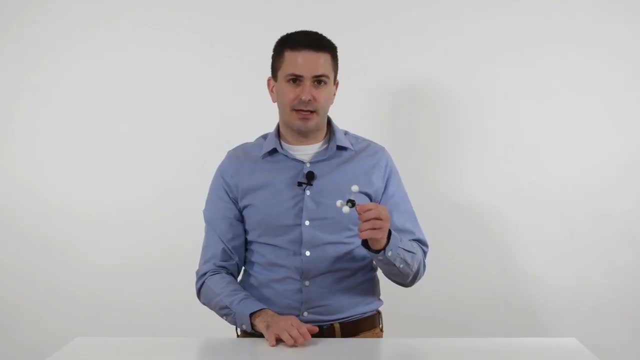 students on their laptops or tablets. Lessons will also be accompanied by video demonstrations which can be used to efficiently train teachers in our methodology. A video series of all our lessons could be used to reach homeschoolers, college students or any adult interested in learning. 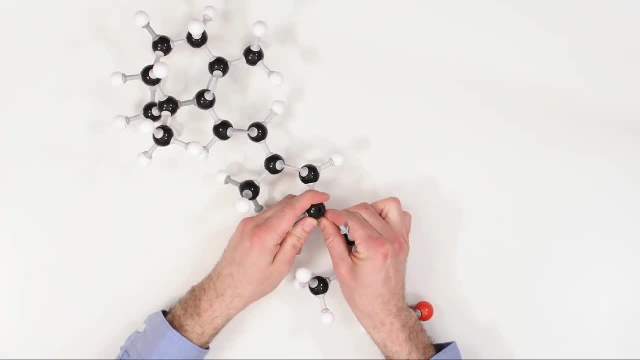 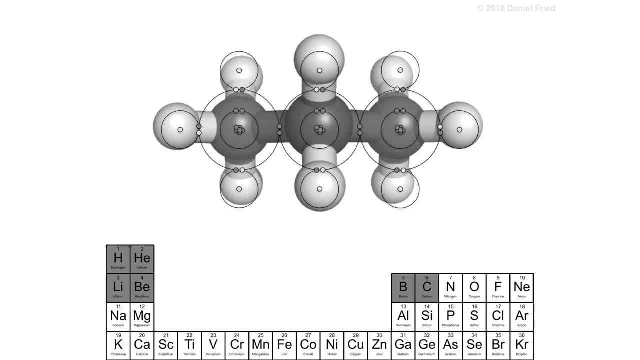 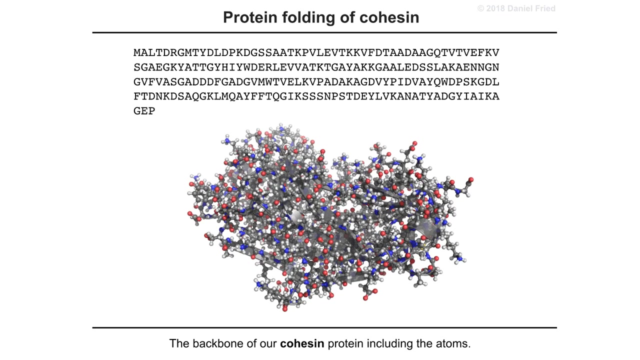 directly from us. This model building activity is about understanding how vitamin A works. Our animated lessons begin simply helping students understand how atoms come together to make small bonded structures like this propane molecule. These simple concepts set the stage for understanding how complex molecular structures work. This lesson is about the link between amino acid sequence and protein.